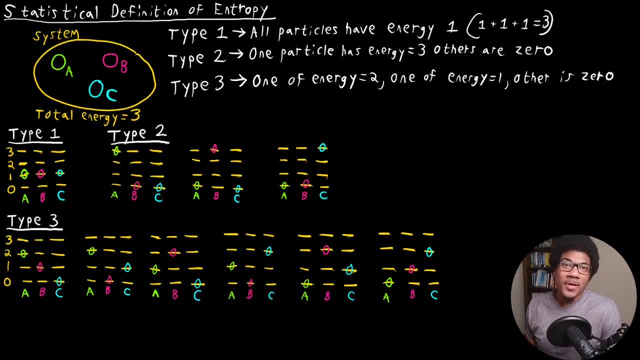 In this video we're going to discuss the statistical definition of entropy. Up until this point, we've discussed entropy as the dispersal of energy right, how energy is dispersed in different processes. That's a very macro level explanation of entropy. In order to have any sort of insight onto entropy on a micro level, we really have to look at this statistical definition. So we're kind of going to start with this. this figure here, which really the basis of this is that 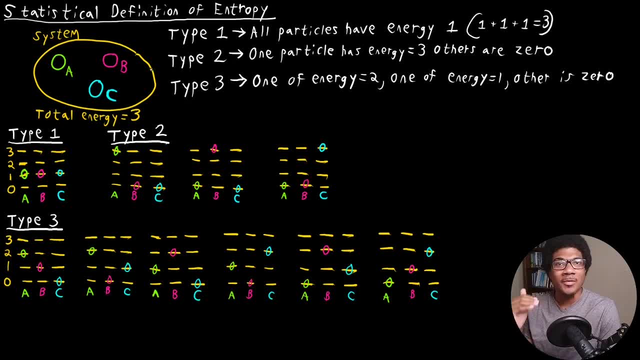 any atom or molecule can only occupy certain energy levels, And this is a result that we'll talk about more when we start talking about quantum chemistry, But right now, hopefully, you have a little bit of an appreciation for the fact that any assortment of atoms or molecules has a particular energy right. So let's take this example system that is a collection of three different particles, particle A, particle B and particle C, And we'll say that the total energy of this system 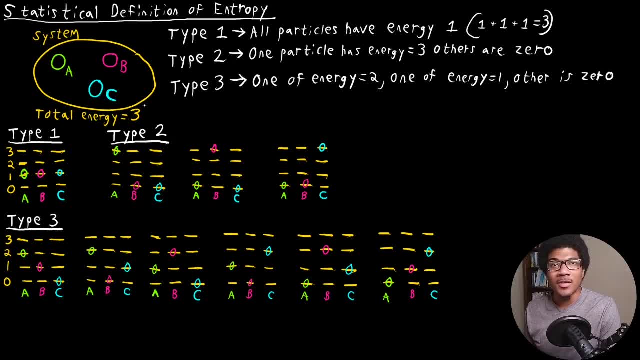 that is, a collection of three different particles, particle A, particle B and particle C, And we'll say that the total energy of this system, this collection of particles, has a total energy of three. Now, each of these individual particles can occupy different energy levels, from zero all the way to three, So they can have no energy. 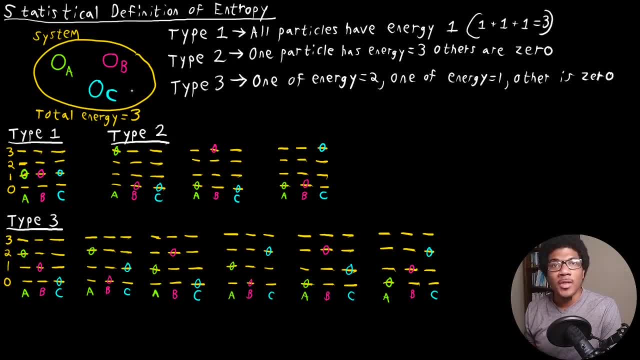 or, at maximum, have an energy of three. If we think of a system being distributed in this fashion, we can imagine three different ways that we can distribute these particles and still get a total energy of three. So the first way that we can think about: 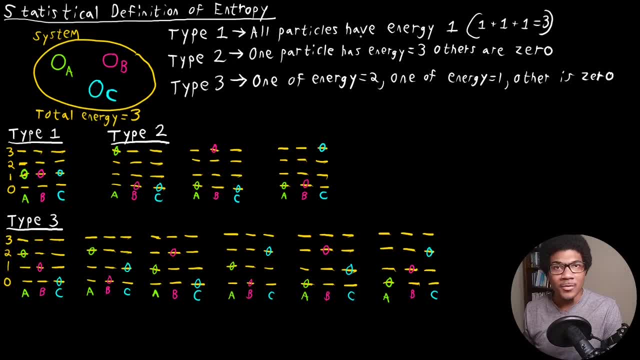 distributing these particles' energies is if all the particles have an energy of one. If they each have an energy of one, they contribute one to the total energy. you get a total energy of three. The other way you can think about it is: if, well, if one particle has an energy of three, 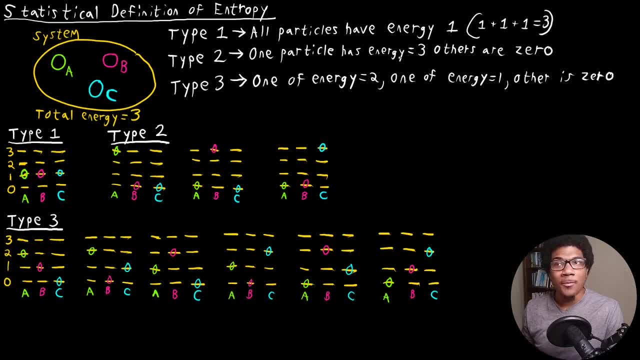 and the other particles have an energy of zero. And the last type is type three, where one of them has an energy of two, the other has an energy of one and the other has an energy of zero, right? So each of these? 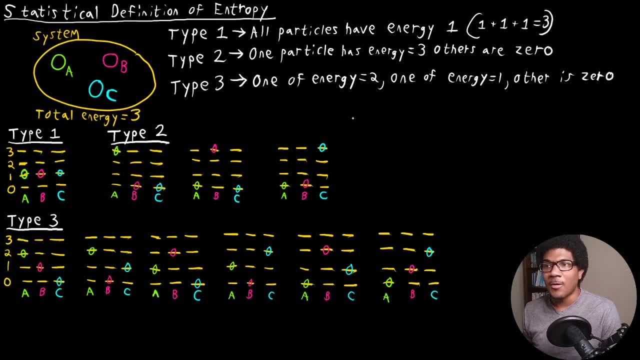 these different distributions of energy are called microstates. right, So we can distribute these particles in different ways to get the same energy. These individual distributions are called microstates. So I've drawn a visual representation of all of the different microstates of different 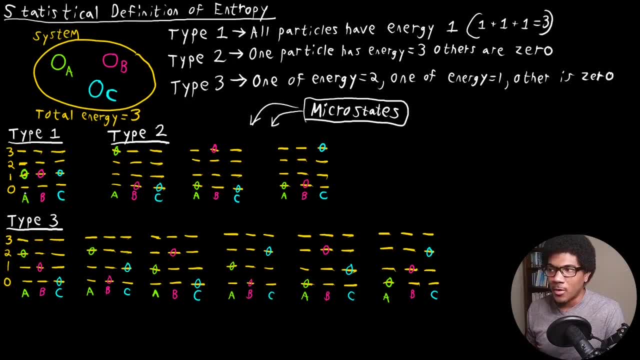 types below right. So we see type one here, where all of them have one. Note that in type one we only have one microstate right. So for for type one, there's only one microstate Right. There's only one way to distribute the particles. in that fashion, Each one of them has one. 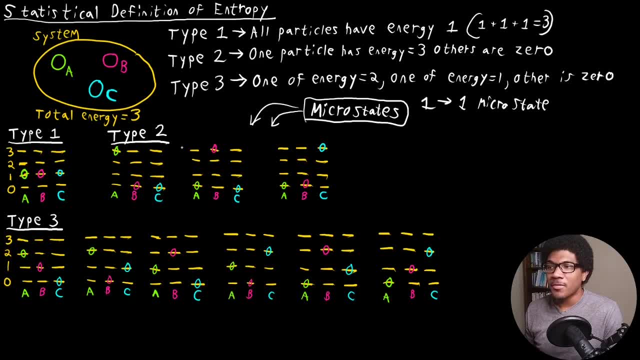 There's only one way to do that right. However, for type two, we start to see that we can have multiple different microstates. So the first microstate that I have here for type two, particle A, has an energy of three, and the rest of them have energy of zero. For the 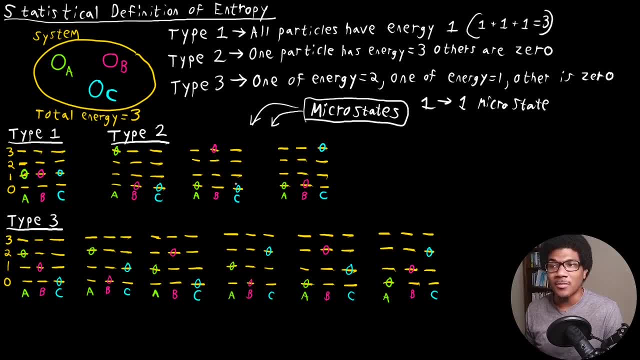 second one: particle B has an energy of three, the rest are zero. And then the last one is where particle C has an energy of three and the rest have zero. This gives us three total microstates, right? So for type two we can have three microstates, right? So whenever you have, 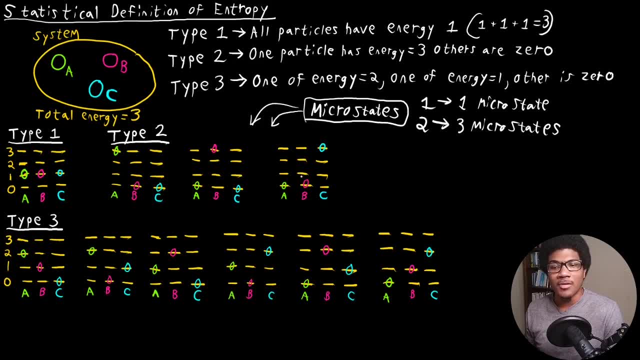 multiple microstates that give you the same energy. these are called degeneracies. So we're going to use the letter W to denote degeneracy, right? So we would say that type two distributions are threefold degenerate, which just means that we have three different ways. 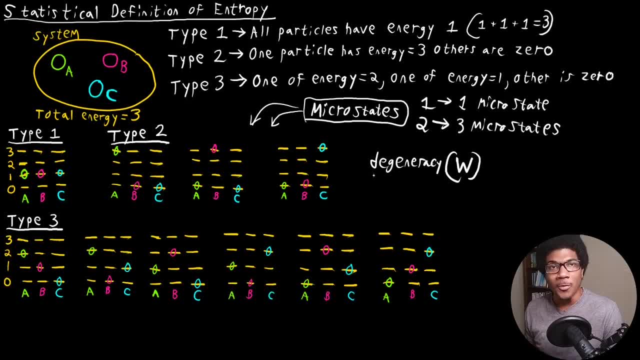 to distribute the particles and still get this same total energy representation right. So degeneracies are just a number of ways of achieving the same energy right. So number of ways, number of ways of achieving a given energy state right, That's degeneracy. 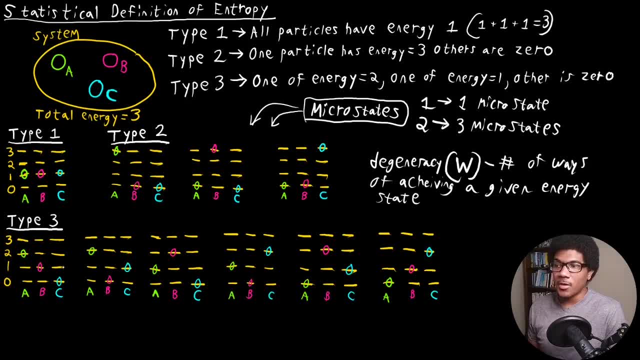 So now, if we go to type three, what we notice is that there's six different ways that we can distribute the particles. with a type three distribution right, Where one of the particles has energy two, one of them has energy one and the other has energy zero, There's six. 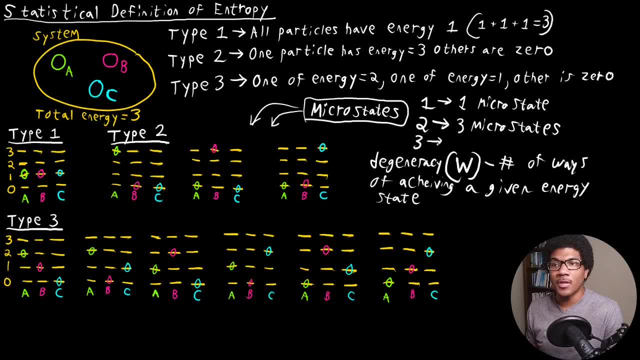 different ways of doing that. So type three is going to have six microstates, right. So what the statistical definition of entropy is really based on is how much degeneracy you have in a given configuration. The higher the degeneracy, the higher the entropy. 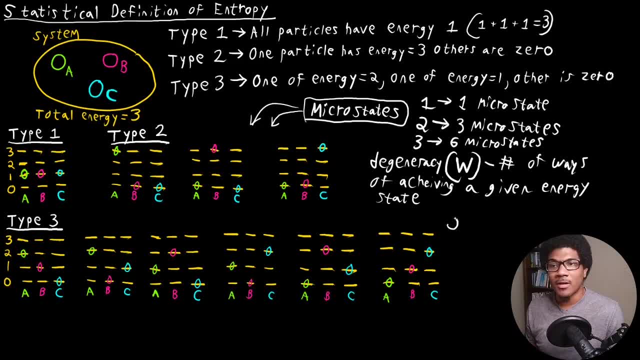 And it's governed by the Boltzmann equation, which basically says that the entropy is going to be equal to K, the Boltzmann constant times, the natural log of the degeneracy, So the natural log of W right? This is the Boltzmann equation for entropy, right. 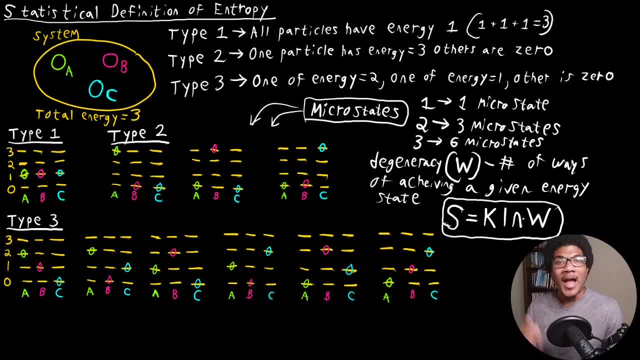 So basically, the higher the degeneracy, the higher the entropy. right. And this gels well with our definition of entropy as the dispersal of energy. We say that the more dispersed energy is, the higher the entropy is right. So the same thing here: the more ways you can disperse, 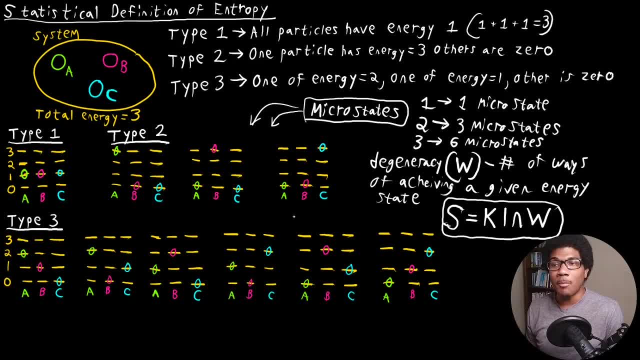 the particles or distribute particles in these different microstates, the higher the entropy is going to be, And we can kind of think about this through the lens of the second law of thermodynamics as well. So if I were to ask you which type, if you were to throw these in a bag, 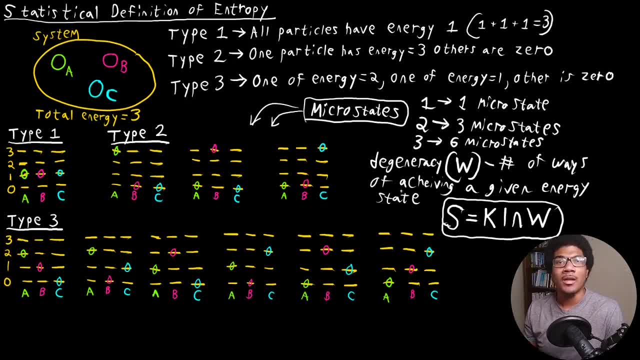 and randomly pick one out. randomly pick out a microstate. which one would you most likely be picking out of that bag? right, You would be picking most likely a type three distribution if you were to just randomly select one right Now with this one, it's still rather likely that. 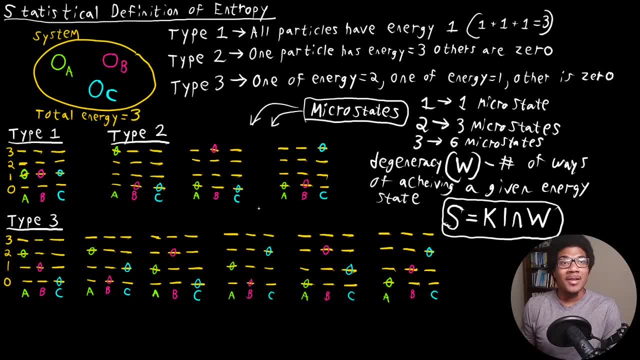 you get a type two or a type one distribution, but you can imagine how this starts to become much more likely as you go to larger and larger scales. Think about a small solid that has Avogadro's number worth of atoms in it. right Now you start to think about. 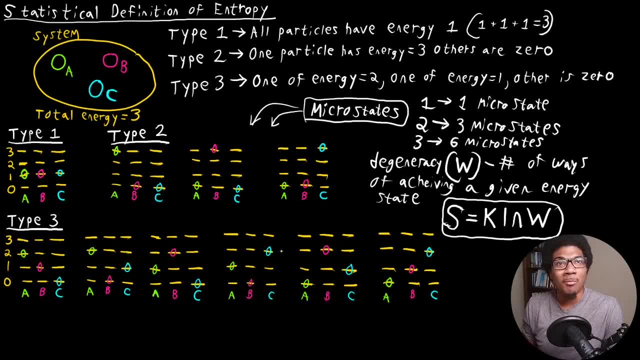 okay, if there's whatever distribution is most dispersed, whichever one has the most possible microstates, that's going to be the one I'm most likely to find this system in, right? So that kind of gels with the second law of thermodynamics, right?